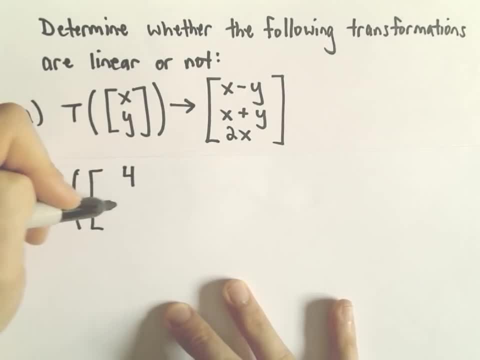 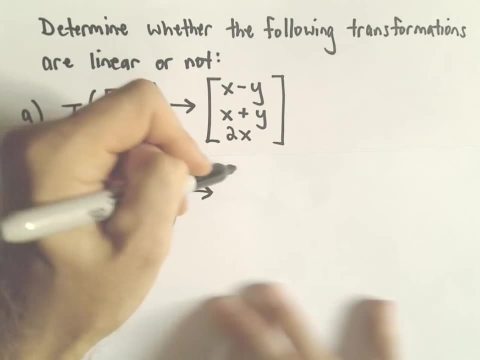 This first example. You know, if we started with the vector 4, you know 15.. So that's a vector in R2.. It says under this mapping: all it says is take the first component, subtract away the second component. 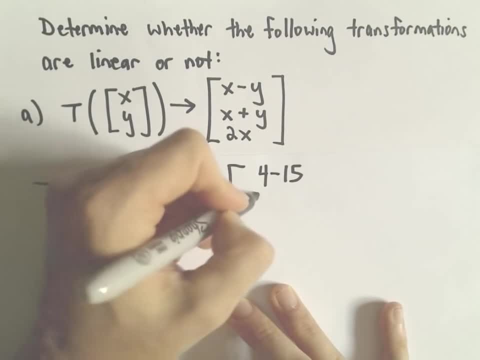 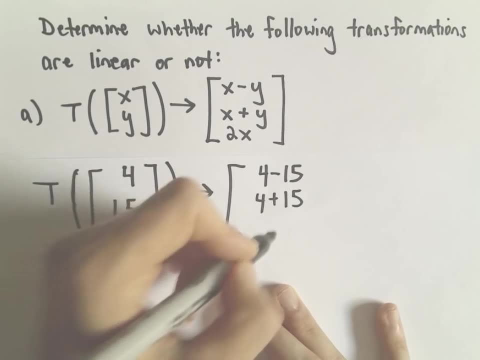 So we would have 4 minus 15.. Then it says: add the two components together, 4 plus 15.. And then it says: take the first component and multiply it by 2. So we would get 2 times the first component. 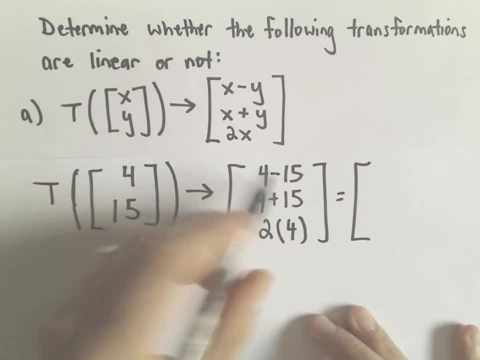 which is 4.. And well, 4 minus 15,, what is that Negative 11.. 4 plus 15,, that's 19.. And 2 times 4, that's going to be 8.. So, under this transformation, 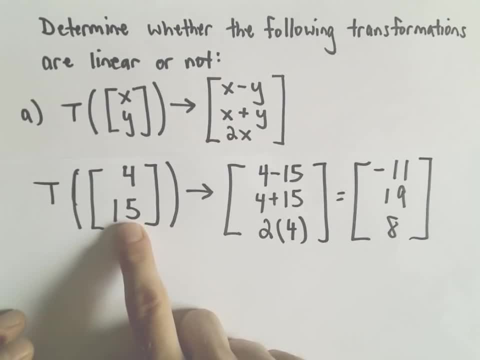 it's going to map the vector with components 4, 15 into R3, and it's going to give us the vector with components negative 11,, 19, and 8.. So again, nothing crazy there. That's all it is. 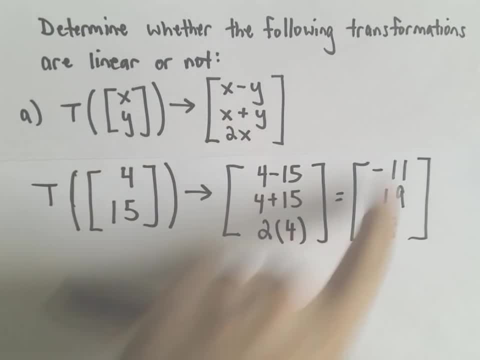 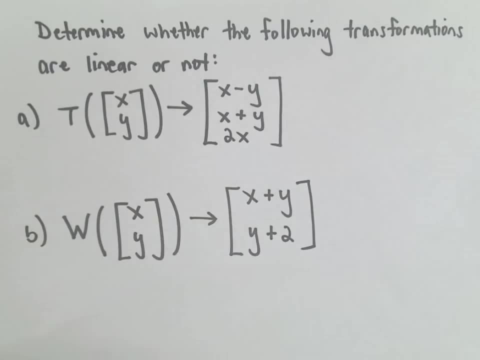 Just taking one vector: It has some rule, It has some rule associated with it and it produces a new vector. All right, let's decide if this transformation is linear or not. And oftentimes again, when you're trying to prove something or justify something, 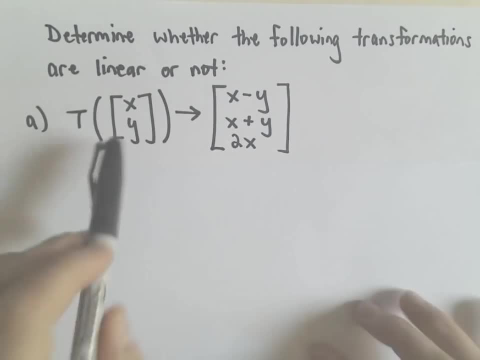 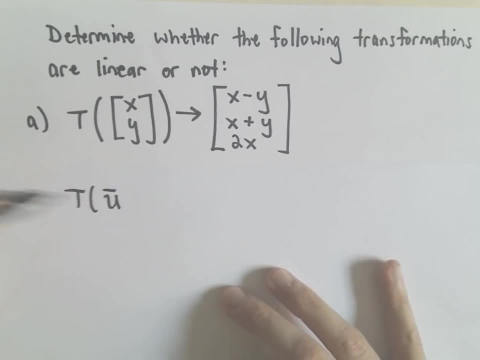 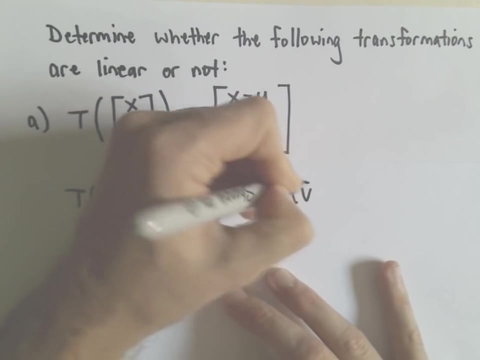 it's just a matter of using the definitions. So I'm going to break this one up into two videos and part one will justify this first condition. So just T of U plus V. does that equal the transformations? It's just a matter of how many vectors you have individually added together. 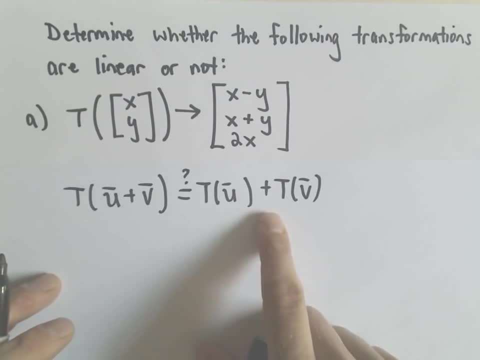 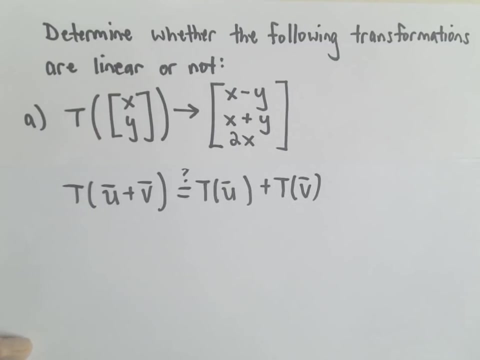 So obviously if this first condition doesn't hold, there's no point in showing the second condition about the scalar multiplication, because obviously if one condition doesn't hold it's not linear. But if this one holds, we'll go back and show that the scalar multiplication does or doesn't hold. 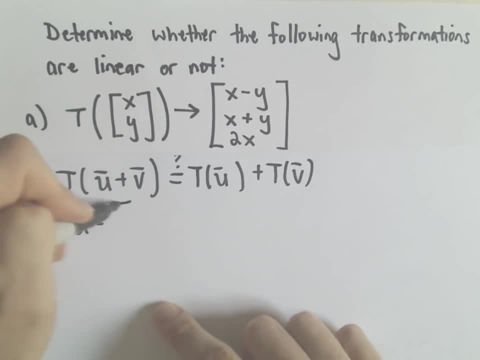 Okay. so the way I'm going to do this is: I'm just going to pick some vectors. I'm going to let vector U have components A1, A2.. We'll let vector V have components, let's say, B1 and B2.. 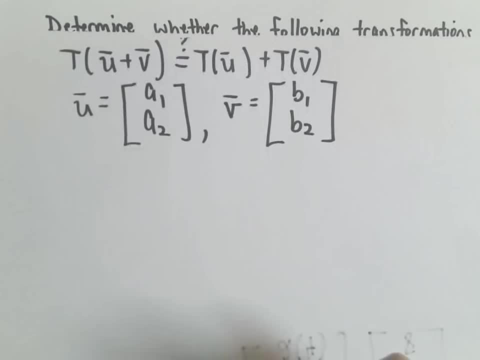 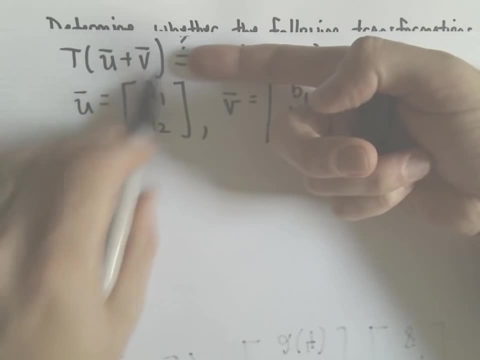 And now I'm just going to start applying things individually. So if we take T of U plus V, so I'm going to find an expression for this left side. I'm going to get an expression for the left side, Then I'm going to come back, figure out an expression for the right side. 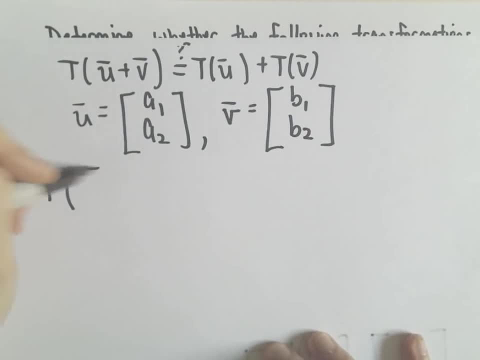 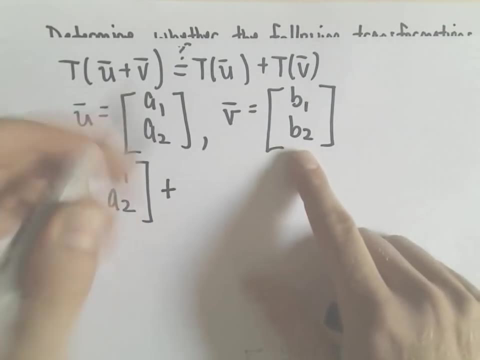 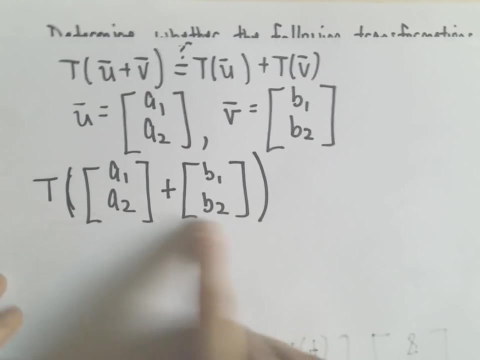 and we'll just compare them, see whether or not they're equal. So vector U, that's A1 and A2.. Plus vector V, which has components B1, B2.. Okay, so again we know how to add vectors together. 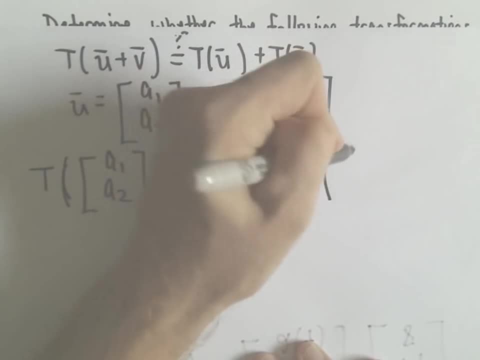 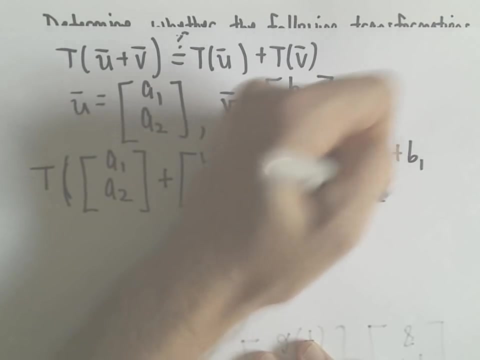 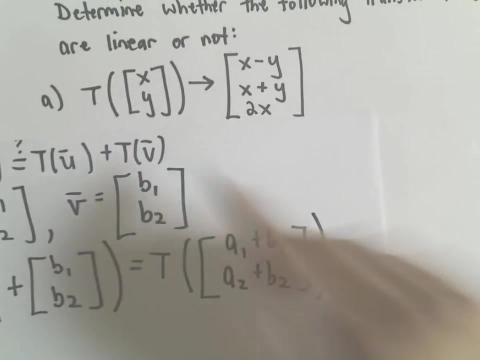 We just add them a component at a time, So we would get A1 plus B1, and then we would get A2 plus B2.. All righty, now I'm going to go back to my actual rule here, and this is the rule. 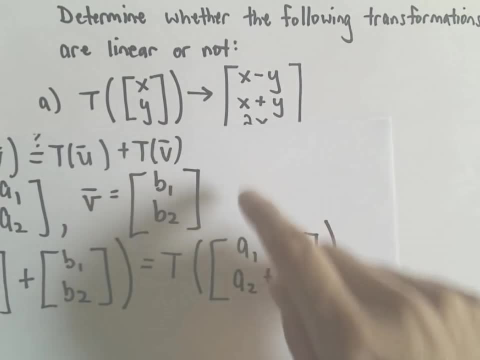 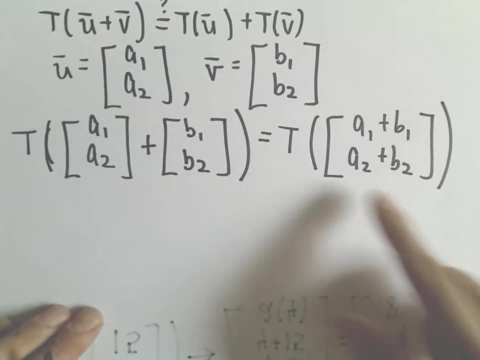 This tells us what happens in this transformation. So again, take the first component minus the second, add them together and then multiply the first component by 2. So if we apply that transformation, it says again the first thing that happens. 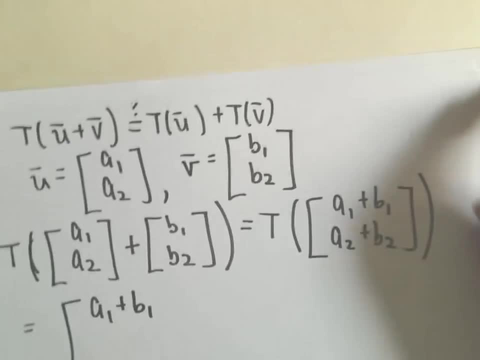 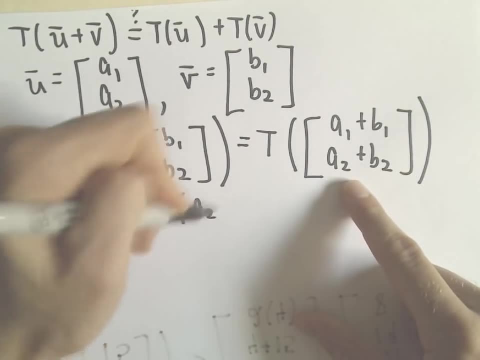 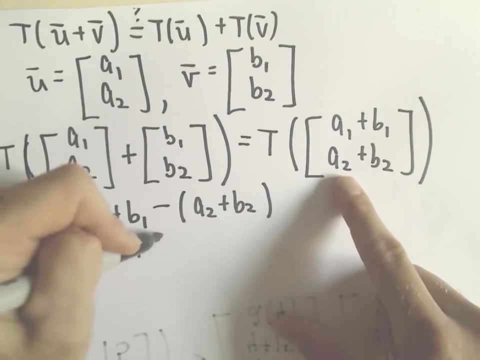 we said was we take A1 plus B1, we take the first component. Now I've already forgotten Subtract away the second component. so minus A2 plus B2.. The second one says A1 plus B2.. So we're going to just add the first component, A1 plus B1,. 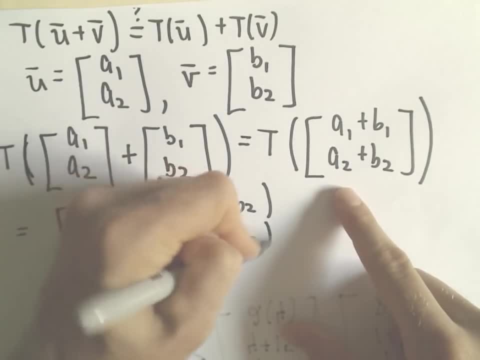 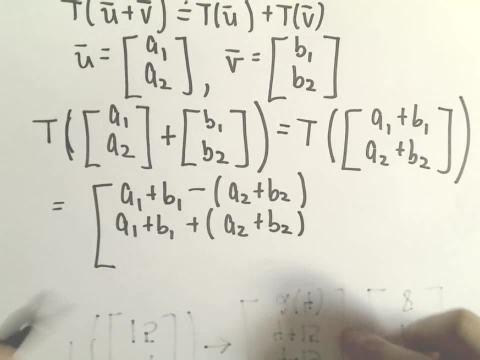 to the second component, A2 plus B2.. And then the third condition said: take whatever the first component was and multiply it by 2. So we'll have 2 times A1 plus B1. And of course you could simplify this down if you want to. 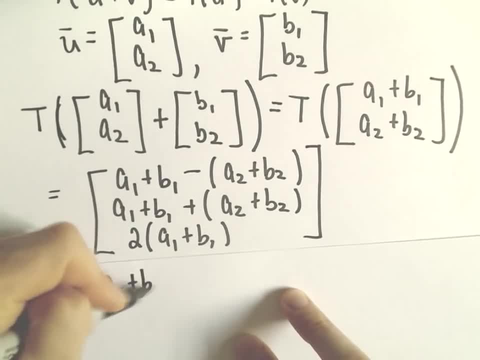 So if we simplify it down a little bit, we'll have A1 plus B1.. Minus A2, minus B2. And then it looks like we'll just have, I guess, A1. We could reorder them- Plus A2 plus B1, plus B2.. 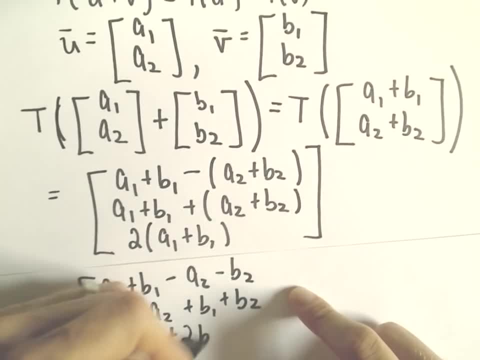 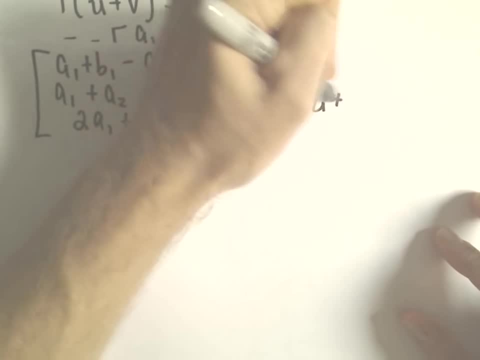 It doesn't really matter. And then we'll have 2A1 plus 2B1.. Okay, so this is what we got when we summed the vectors first and then applied the transformation, So we'll come back to that in just a second. 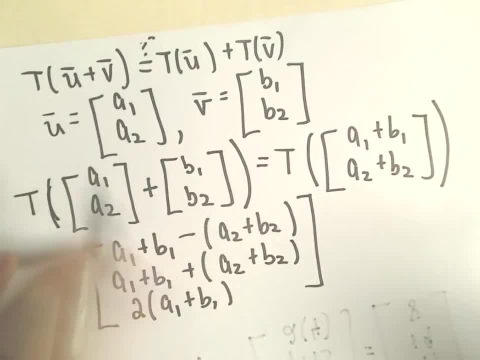 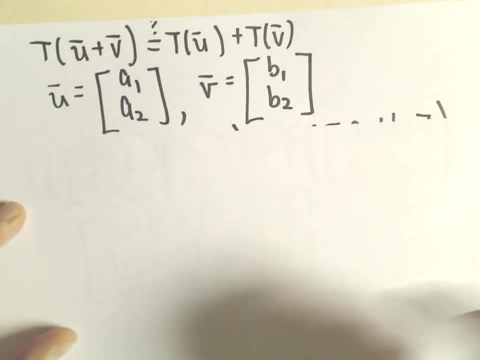 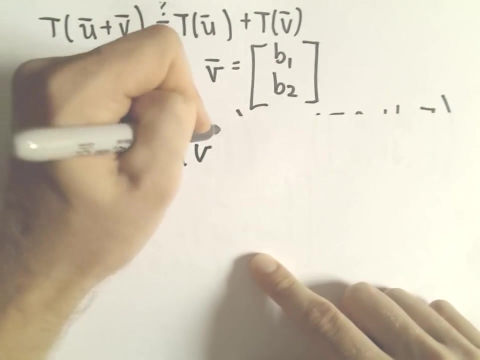 So now, we just figured out an expression for the left side, Let's figure out an expression for the right side as well. Okay, so now we'll figure out an expression T of U plus T of V- Thrilling stuff, But again, this is important. 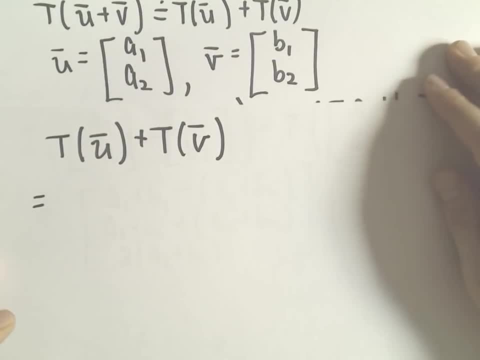 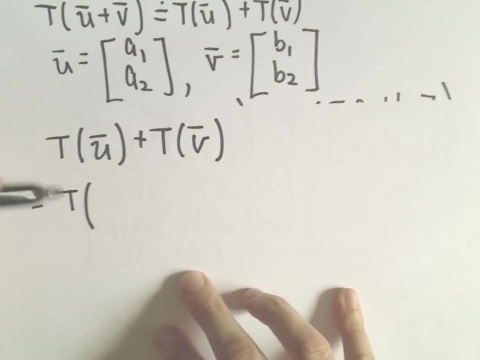 Linear transformations get used all the time, Definitely useful stuff in linear algebra. And then also a good way if you're kind of learning proofs again is just how to apply definitions. So we'll apply the transformation to vector U. So A1, A2, we'll do that one. 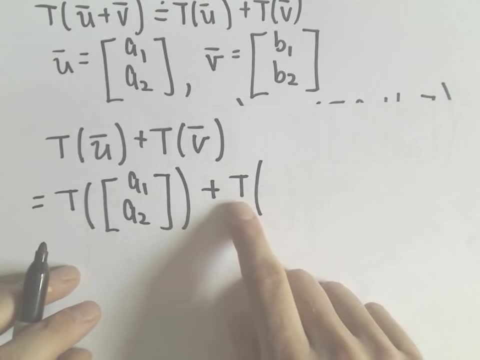 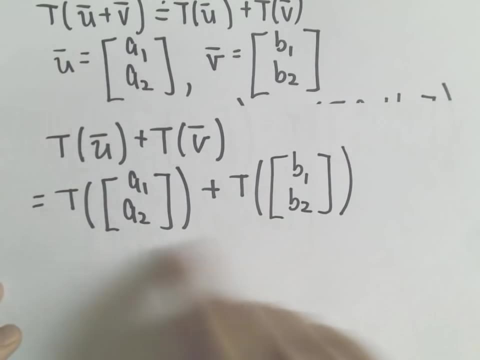 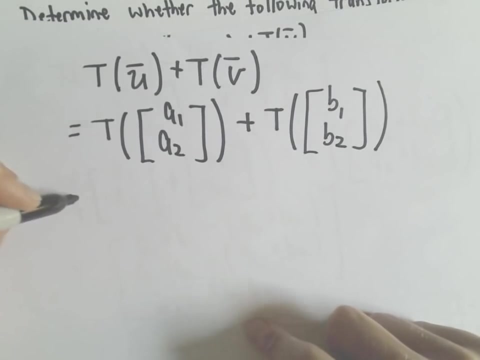 And then we'll add to that whatever we get after we apply the transformation to vector V. Okay. so now, again, I'm going to use my little rule that we started with, Okay. so it says: subtract the second component from the first. 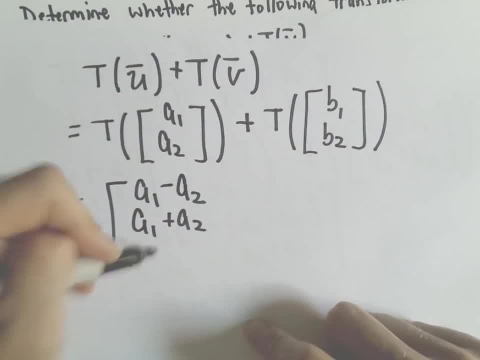 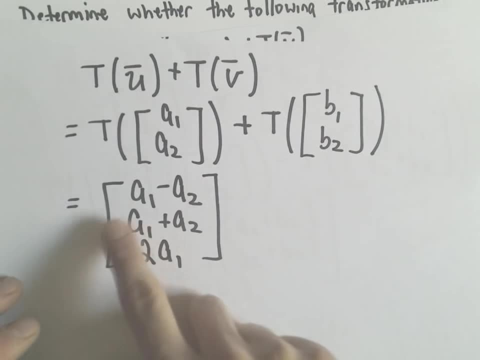 It says: add those components together, And then it says: take the first component and multiply it by 2.. So if we apply the transformation to our first vector, we'll just have A1 minus A2, A1 plus A2, 2A1.. 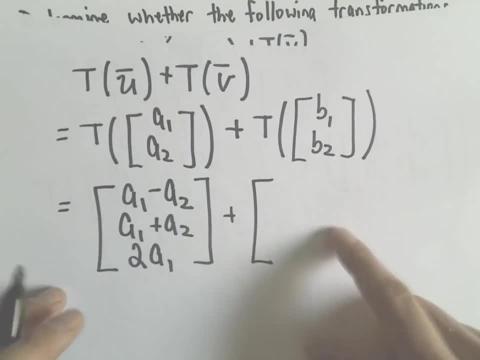 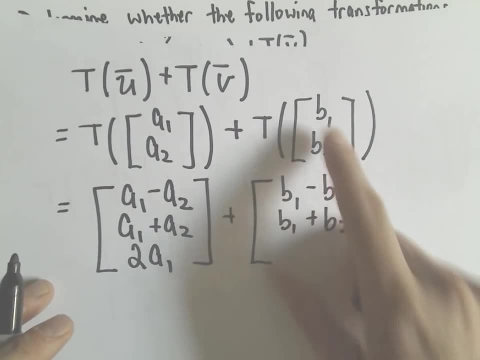 We'll do the same thing. We'll apply the transformation to our second vector, So we'll get B1 minus B2.. We'll get B1 plus B2.. And then it says: take the first component and again double it. 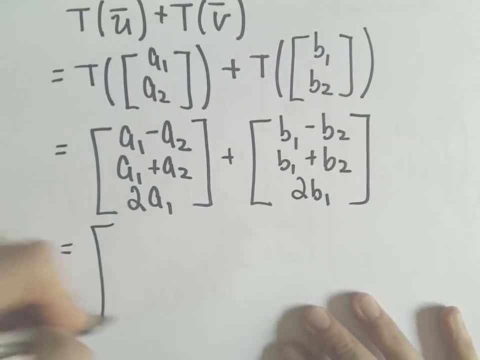 And okay. so again we know how to add or subtract vectors. We just do it a component at a time. So A1 minus A2 plus B1 minus B2.. We'll have A1 plus A2 plus B1 plus B2.. 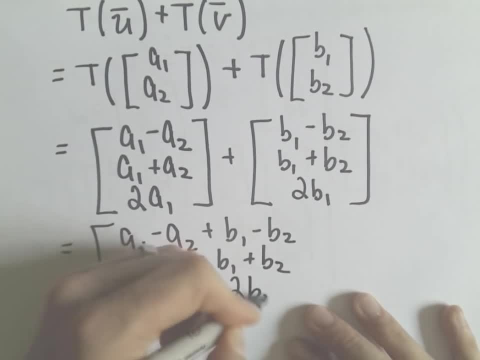 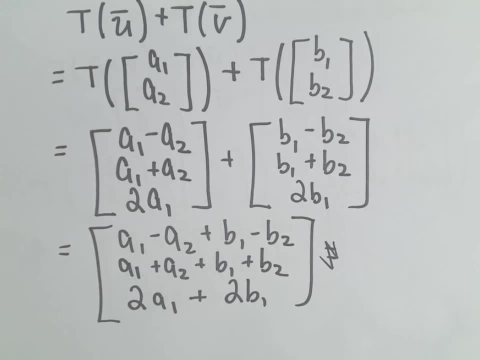 And then we'll have 2A1 plus 2B1.. And again, this is the right-hand side of that expression. So let's see, Let's compare it to what we had just a second ago and see if those are in fact equal.